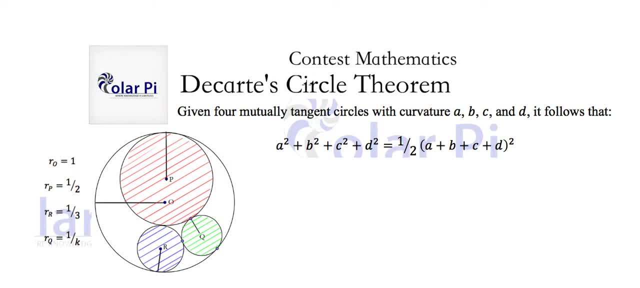 Hey guys, welcome. Yeah, so in this video I'm going to talk about Descartes Circle Theorem. So this will be the first of many videos under Contest Math, And whether we're talking about a famous math contest like the AMC or the AIME, or just your local math contest, you know that. 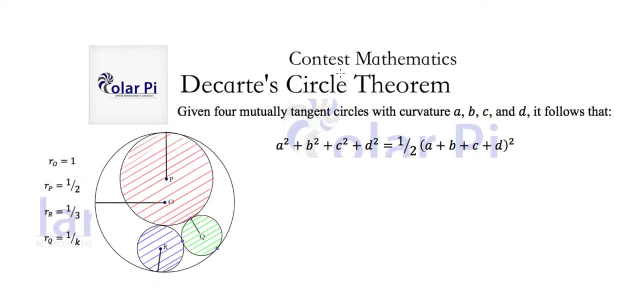 competition. math is all about obscure theorems that are not normally covered in the classroom, And so that will be the case with all of the theorems I present under Contest Math. Now here, Descartes Circle Theorem says this, which is that if we've got four mutually tangent 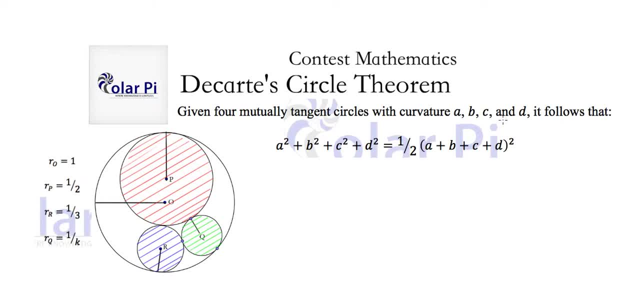 circles with curvatures A, B, C and D, then this equation has to hold true. And, don't worry, curvature of a circle is simply one over the radius of the circle, And so an application of Descartes Circle Theorem will be like here in this example, where we're going to find the 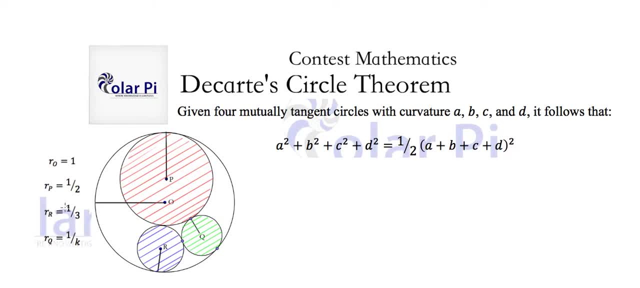 radius of circle Q from knowing the radii of the other three circles, and clearly our four circles are mutually tangent and therefore we can apply Descartes circle theorem. yeah, okay, cool. so first we start the solution by calculating the curvature of the four circles. so if we call the curvature of a circle o the biggest circle, if we call its curvature a, then 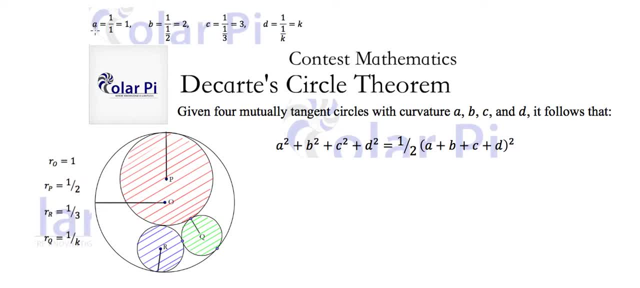 we know, the curvature is one over the radius, so for circle o will be one over one, which is one, so the curvature of circle o, our biggest circle, is one. and then the curvature of circle p will be one over one half or two. and notice, we've called the curvature of circle p b and then the curvature 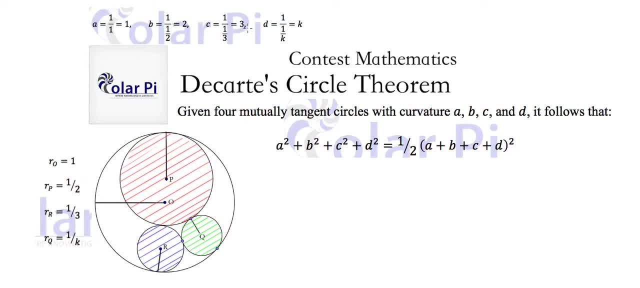 of circle r is one over one third or three, and we've chosen to call the curvature of circle r c. and the curvature of circle q is going to be one over one over k, which is one over one third or two, and then we've chosen to call the curvature of circle r. 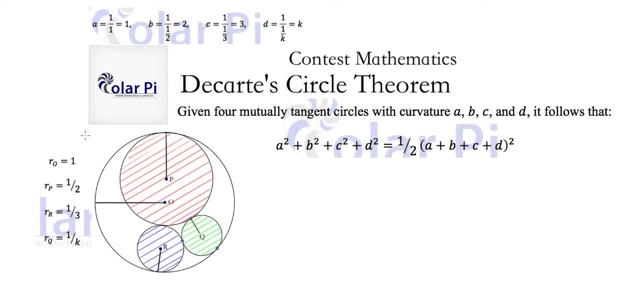 is K, and so it's the radius of circle Q that we don't know, and therefore we don't know its curvature either. we just know that its curvature is K. notice that I deliberately constructed this example so that the curvatures were going to be nice integers, right. but such might not be the case with your problem, but still. 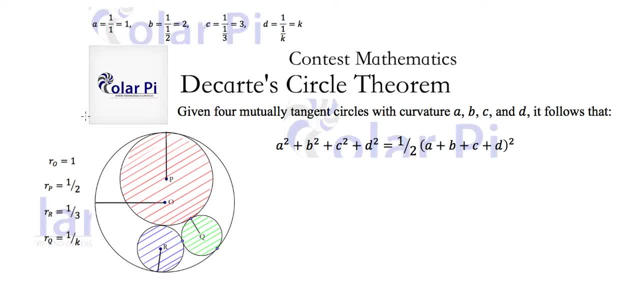 the solution would be: and the same mold is what I'm about to show you. cool, all right. now that we've got the curvature is ABC and D of our four circles are ready to go plug into this formula to get this equation right. okay, cool, now we. 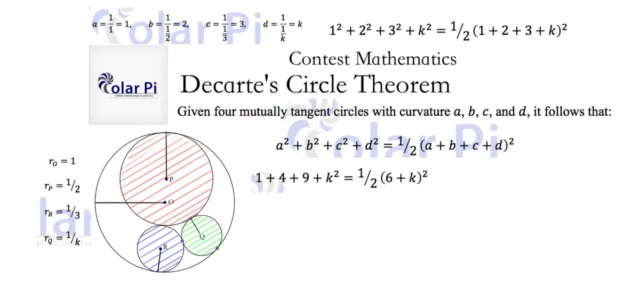 simplify this equation and yeah, and that just requires that you know like 2 squared is 4 and 3 squared is 9 and stuff. and then on this equation, if we simplify it a little bit more, we can write: the left-hand side is 14 plus K. 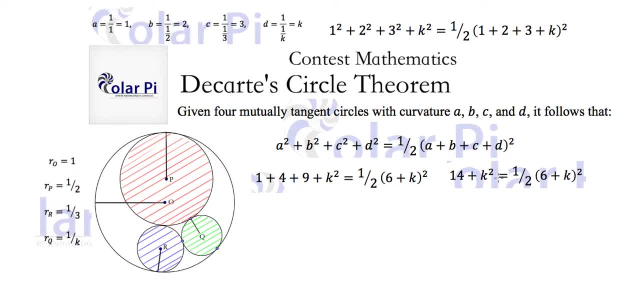 squared and next we're gonna multiply this equation on the sorry y'all- on both sides by 2, and if we do that, then we're gonna get you this equation right, like when we multiply on both sides by 2. here, clearly, the 1 half on the right side is gonna go away, and that's why we wanted to do that. 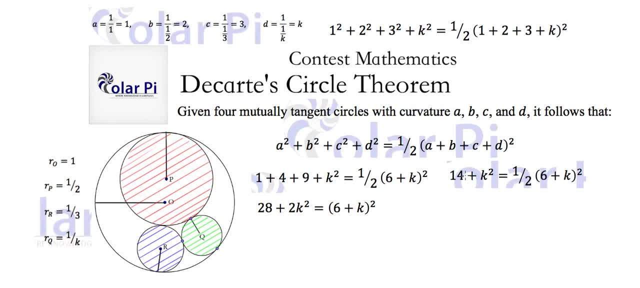 on the left side, we have to multiply both 14 and K squared by 2. therefore 28 plus 2, K squared. yeah, okay, cool. um, now on the right side, here we have that binomial, and if we expand it, that binomial square, I should say, and if we 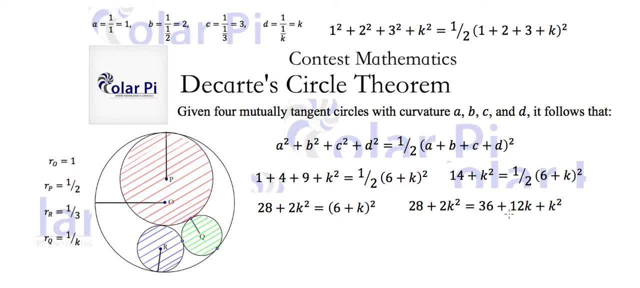 expand it, it's gonna turn out to be this: and if we collect everything on one side, this quadratic will equal 0. then, and it's gonna turn out to be this. you could do it more carefully if you'd like, but it's pretty straightforward: 2 K squared minus. 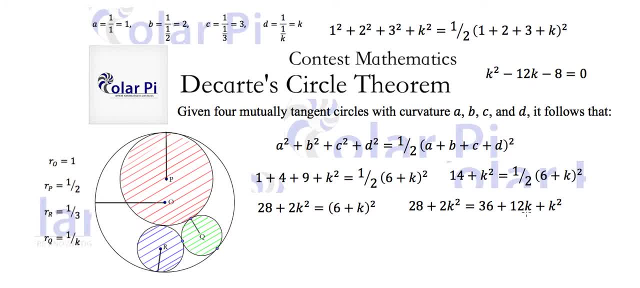 K squared is K squared. and then we bring the 12 K to the left side, so it's minus 12 K, and then 28 minus 36 is negative 8. so we're all good, and of course from here we're gonna solve using the quadratic formula, and so let's make some. 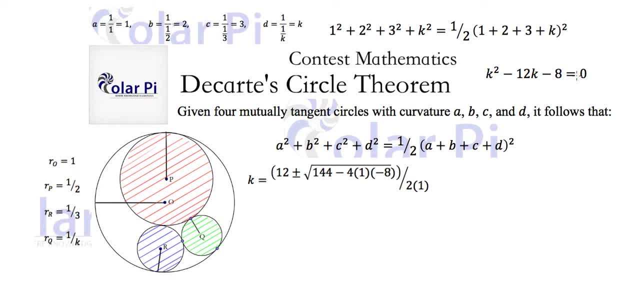 space and plugging into the quadratic formula from here will look like this and simplifying a little bit will look like this, and perhaps the hardest task here in the simplifying steps is to know that 176 can be factored as 16 times 11. 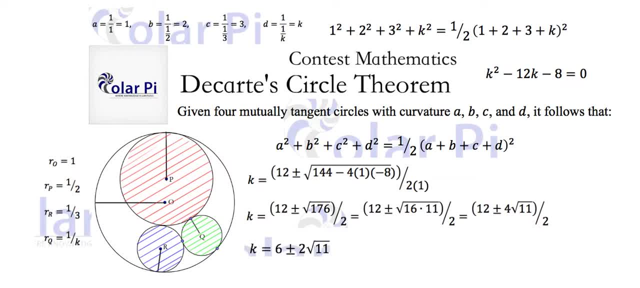 that's a interesting, nice fact to know. but yeah, after all the simplifying, you get to this and now you have to decide: is it 6 plus 2 root 11 or 6 minus 2 root 11? notice: 6 minus 2 root 11 does not make sense because